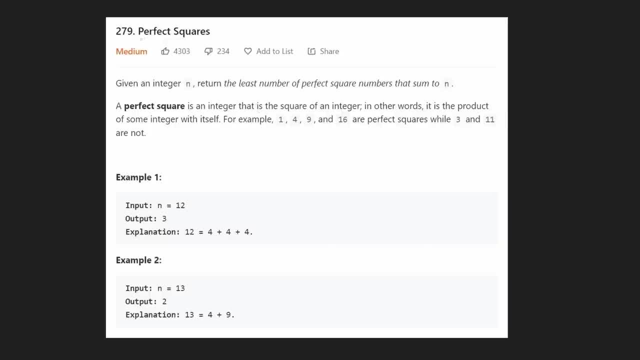 Hey everyone, welcome back and let's write some more neat code today. So today let's solve perfect squares. This is going to be a dynamic programming problem and it's pretty similar to the problem coin change, which I've already solved, and I would say that this is a very similar problem. 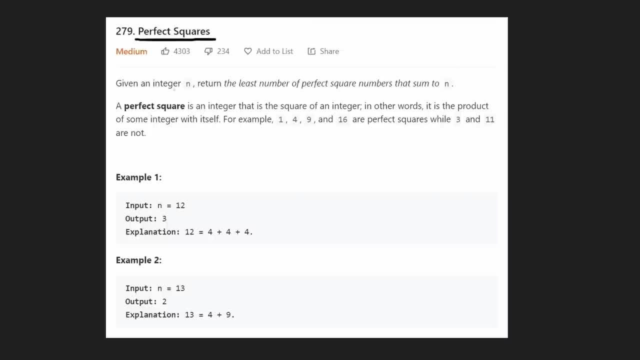 to coin change. It's nearly identical actually. So we're given an integer n. We want to know what's the least number of perfect squares that can sum to this number n. So basically, the difference between coin change and this. In coin change we're given an arbitrary number of coins with 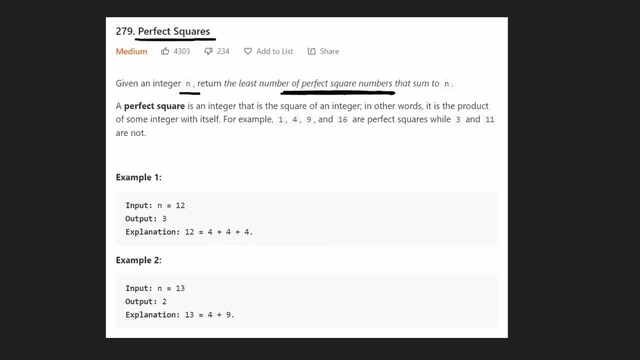 certain values. With this, we're only allowed to use perfect squares. to sum up to the value n And, if you don't recall, a perfect square is just basically a number that has been squared. So, for example, an integer 1 squared is going to end up being 1.. Integer 2 squared is going to end up. 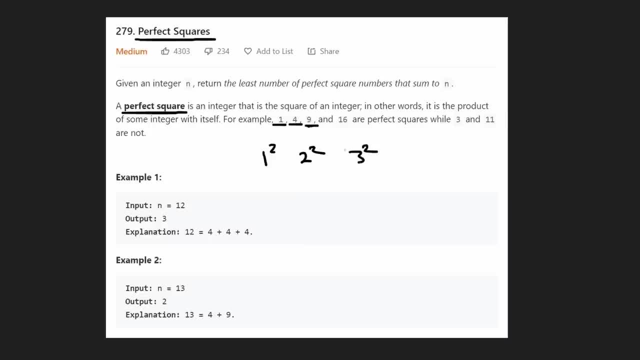 being 4.. Integer 3 squared is going to end up being 9. So on, and so on, and so on. right? So they give us a couple examples: n equals 12.. Minimum number of squares is going to be 1.. Minimum number of: 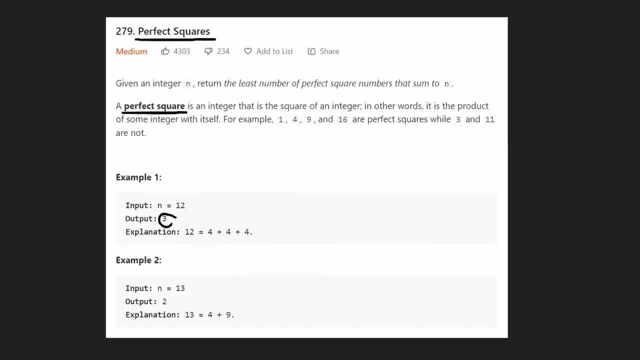 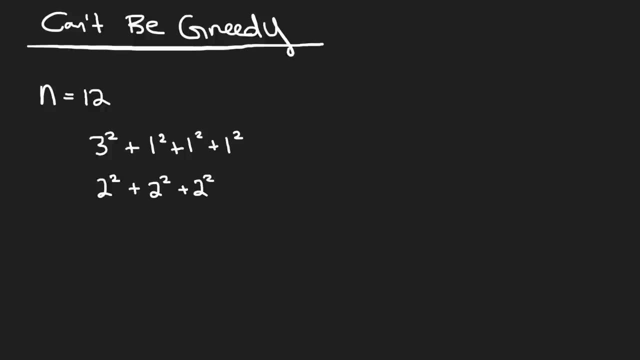 perfect squares is going to be 3.. 4 plus 4 plus 4, that's 3.. 13 is going to be 9 plus 4.. So that's 2 perfect squares needed. So your first idea is probably going to be: can you just be greedy, right? 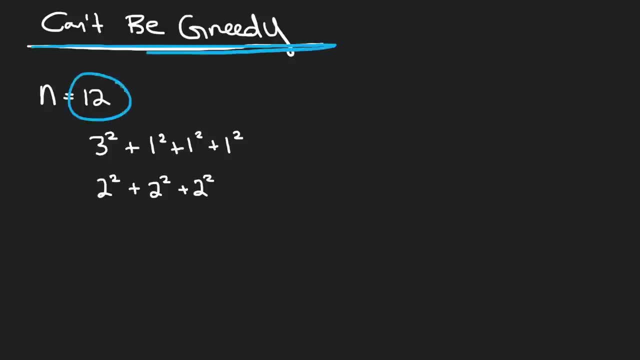 Like: can you just take, for example, 12.. What's the largest perfect square? that's less than or equal to 12, right? Because if we had, like, for example, 5 squared, right, that's going to be 25.. That's too big, right? That's not going to sum up to 12 ever. But let's start with the n, So we're going to. 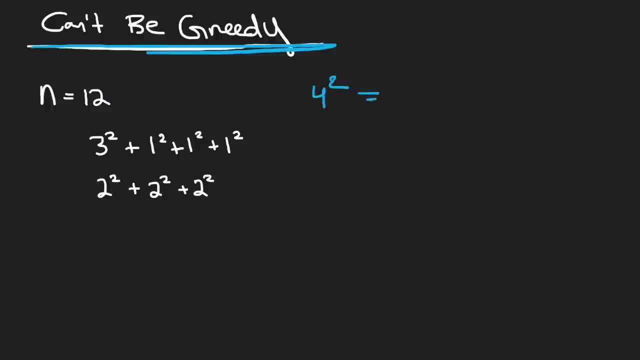 start with the largest perfect square that does Does 4 squared, that's going to be 16.. That's still too big. Then we go to 3 squared, That's 9, right? So we're starting with the biggest perfect square that's available to us. that's less than or equal to 12, right? And so now what we're going to do? 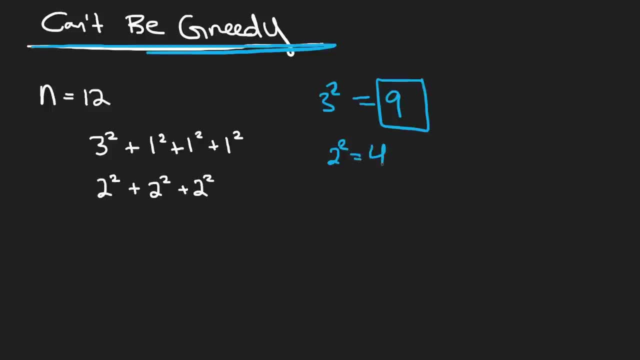 is we're going to try 2 squared right. 2 squared is 4, right. So 4 plus 9 is going to end up being 13, right? So we went too far right, We're trying to get 12.. We went too far right, But I wrote down. 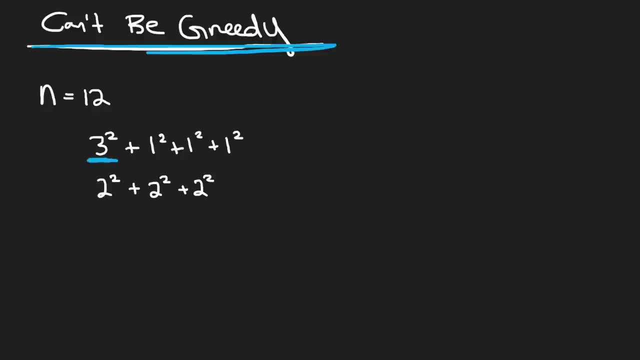 over here. if we started being greedy, right, We started with the biggest one, 3 squared, and then we'd get these values: 1 squared. 1 squared- 1 squared is the only way we're going to be able to sum to 12.. But we notice, if we're not greedy, if we start with 2 squared, for example, that's. 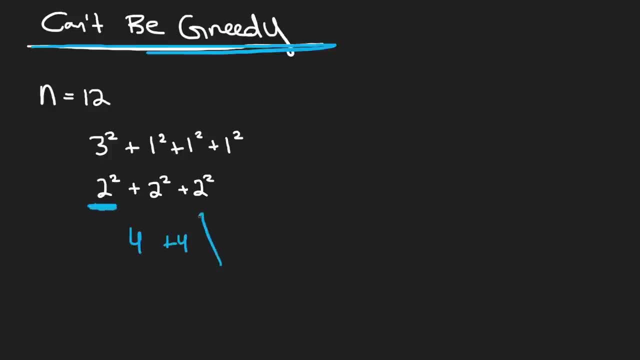 going to be 4.. We get another 2 squared, that's going to be plus 4.. Another 2 squared is going to be plus 4, and that's going to be 12, right? Notice how, with this approach, which was not greedy, 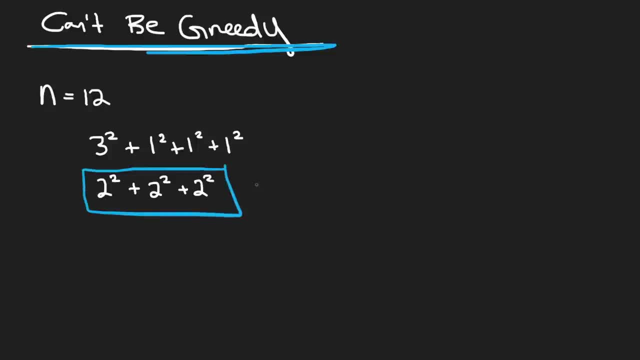 start with the largest perfect squares, But we were able to get it in 3 perfect squares, Whereas when we were greedy over here, we had 4.. So this is not a greedy problem. This is a dynamic programming problem, And I'm going to show you how you can work your way from the brute force. 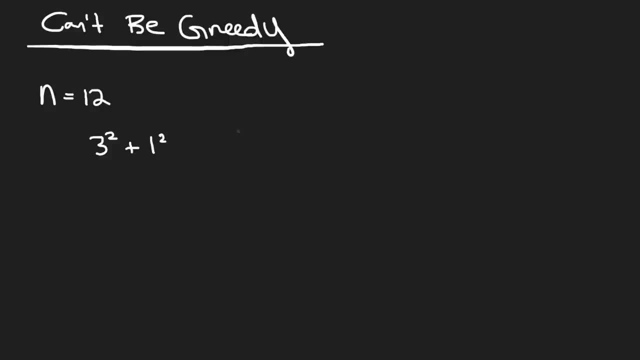 solution to the dynamic programming solution, which is going to be pretty efficient. So what's the brute force approach? usually with dynamic programming problems, Usually a brute force approach is always going to be a decision tree. So let's say we start out with our sum being 0. right, Of course we want our sum to be 12, but initially we're 0. So we have. 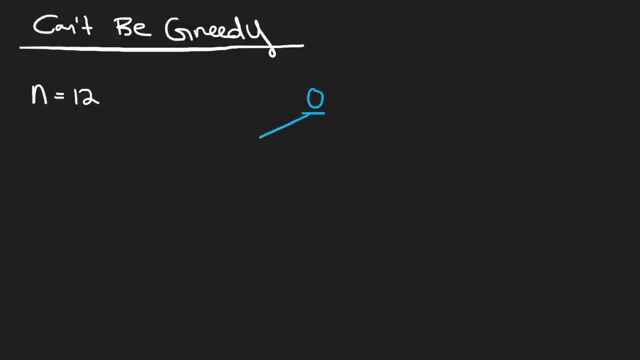 a few branches that we can take. We can start with 1 squared, right, That's one perfect square we could choose. We could start with 2 squared- That's another perfect square we could take. We could try 3 squared, which is another perfect square, And then we would be sequential, right. 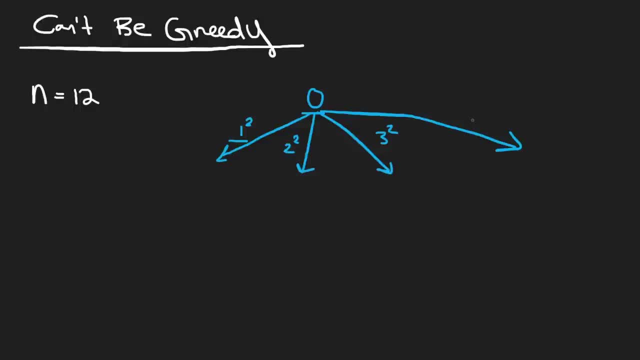 We'd go 1, 2, 3, 4 and just keep going like that until we get to 4 squared. right? What does 4 squared lead us to? That leads us to a sum of 16.. So clearly we went too big right. 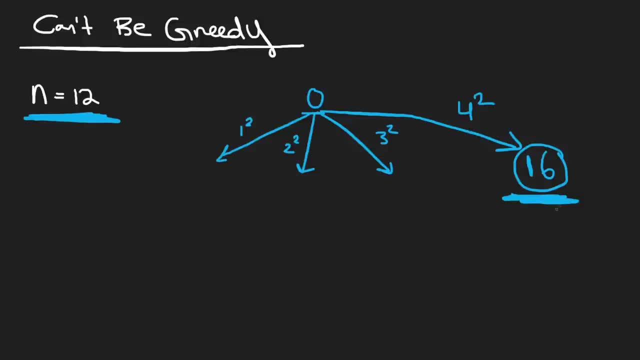 16 is greater than 12.. We went too large, So this is not going to be the path we take. So once we get to this point, we can just stop immediately. We're not going to continue down this path. But with these other three we'll get a sum of 1 of 4 of 9. And so I'm not going to draw the entire. 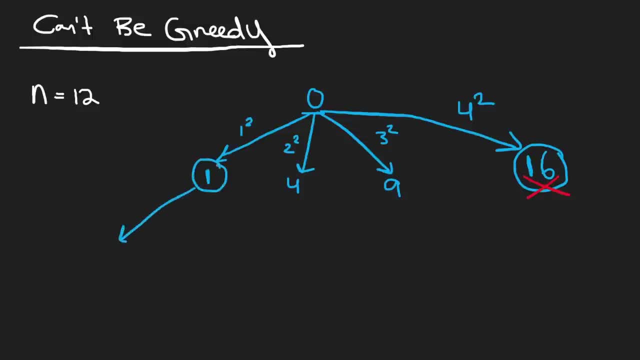 decision tree, but that's basically what it would be right. So, from this 1, we would also have, you know, the same three choices: 1 squared, 2 squared and 3 squared, And that would lead us to sums of 2.. 4 plus 1 is going to be 5.. 9 plus 1 is going to be 10.. So these would be our sums. 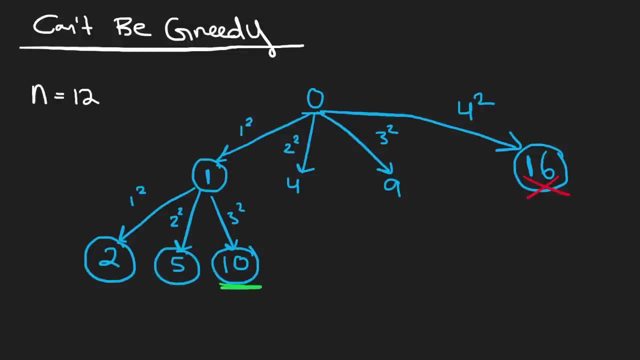 so far And basically you can tell. For example, we got to the sum 10 right. It took us two perfect squares, A 1 squared and a 3 squared, to get to this right. So basically, the height of this portion is going to be the number of perfect squares it took us to get here And the thing you're going. 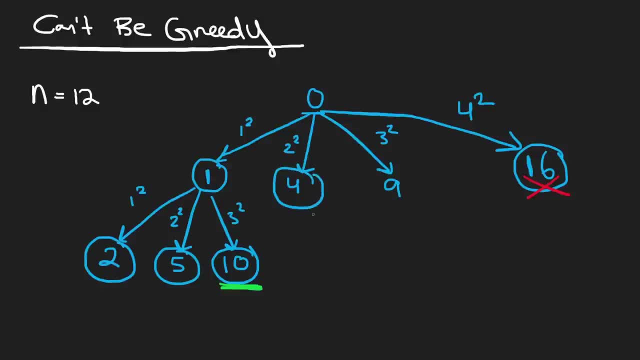 to notice with this decision tree is that there's going to be a lot of repeated work. For example, from here, if we took a 1 squared right, then we'd get 5 again right, But we see that there's already a 5 over here and now we have another 5 over here. So there's going to be a lot of repeated work in. 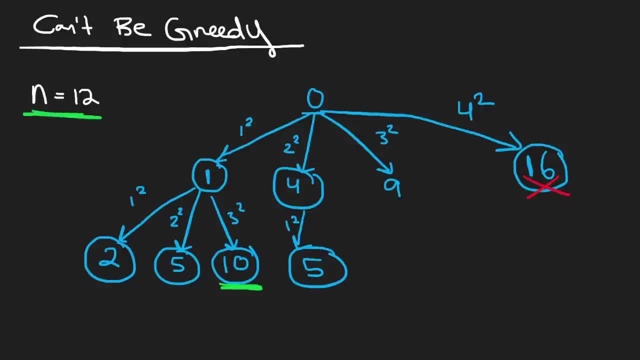 this decision tree And remember: our ultimate goal is to get to this: sum: n equals 12, right, And so we use right. 10 tells us, so far we're at 10.. Our goal is to get to 12, but so far we're at 10.. Here. 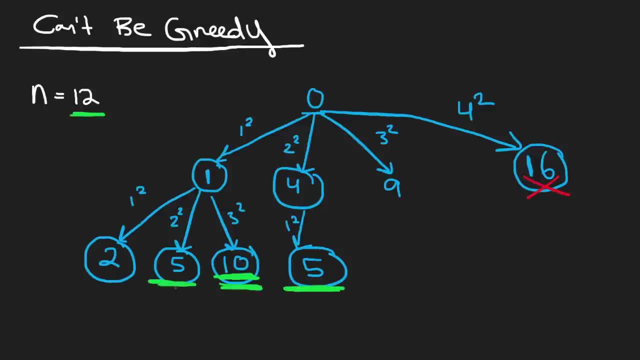 we're at 5.. Here we're also at 5, right? So do we really need to continue down both of these paths? because from here we can see that it took us two perfect squares to get here. From here, it also took us two perfect squares to get here And from here. what we're now trying to determine is if we 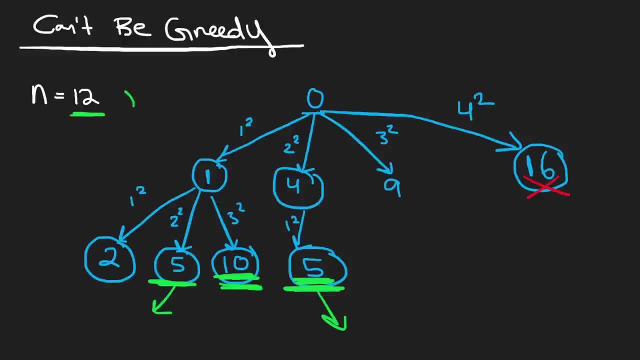 start at five. how many perfect squares does it take us to get to 12.? From the original root, We were trying to determine from zero. how many perfect squares does it take for us to get to 12.? Or thinking about the problem in a different way: once our sum is five, in reality, from here on we're 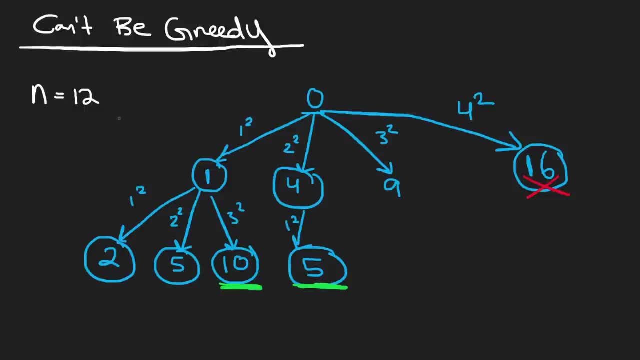 really looking for what's the minimum number of perfect squares, not what it takes to get to 12, because we've already gotten to five, But right now we just want a plus seven to add to this five so that we can get to 12. right? Because when you look at the decision tree, 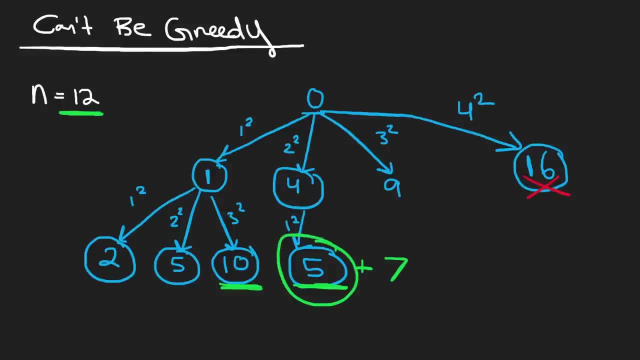 because we've found that to get to five, the minimum number of perfect squares it takes is two, And so we want to know from here: what's the minimum number of perfect squares does it take to get to seven? Then we can see if this is a possible solution. But of course we know that. 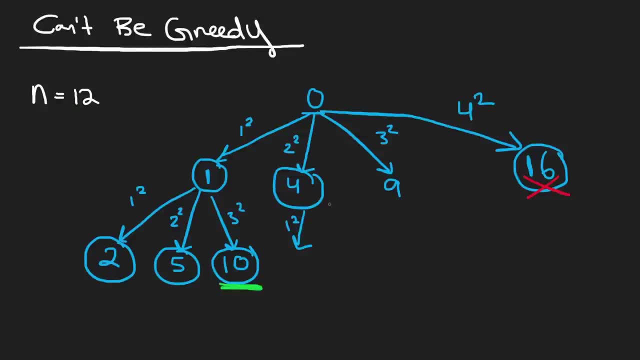 the actual answer is going to be a different path. It's going to be from here, where we take another two squared and we get to a total of eight. And so from here we're looking for what's the minimum number. So we have eight now, right. So we're looking for eight plus four is what's going to. 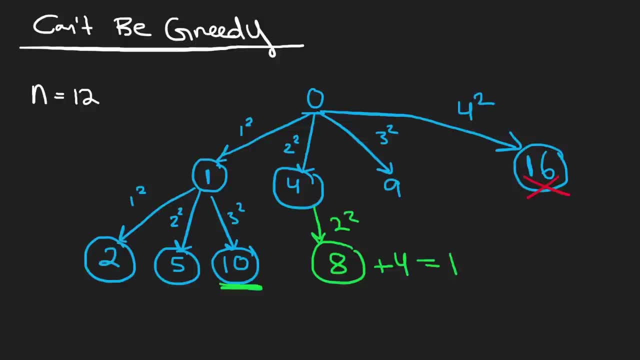 give us 12.. So, at this point, what we're looking for is: what is the minimum number of perfect squares? does it take for us to get to the total of four? And we know that there exists a perfect square that exactly matches four, right? We know two squared is equal to four, So how many perfect? 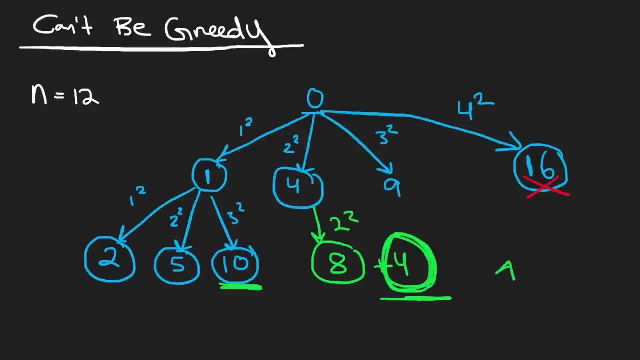 squares does it take to get to four? It takes exactly one perfect square. So we know that that's actually just a given right. It takes a single perfect square. So then we can see that in total it'll with this path. it'll take the minimum number of perfect squares. 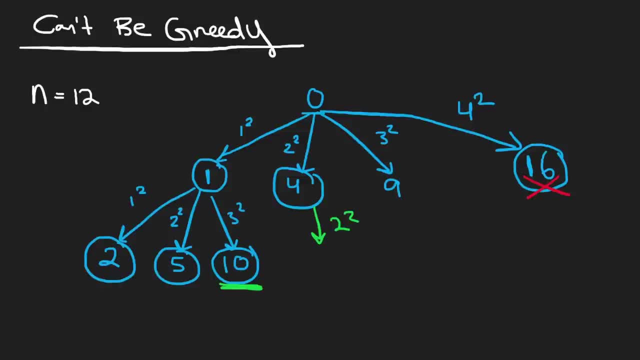 will be three. So let's now try to actually formulate what. what exactly is the sub problem in this case? So we know, we tried, we started at one, two, three, four and we just went arbitrarily high until we got to a value four where four squared was 16, and that was too large than this. 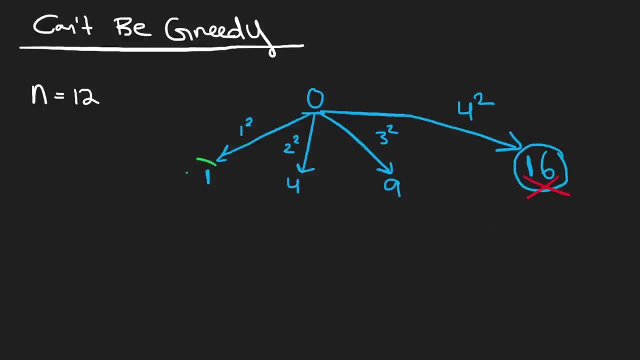 right. So in reality we had exactly three choices: one, four and nine. These were our sums initially. So, along this path, we actually took this n equals 12 and changed the sub problem to actually n equals 11, because we know we've gotten a sum of one so far. we want to know what's the minimum number of perfect squares does it take? 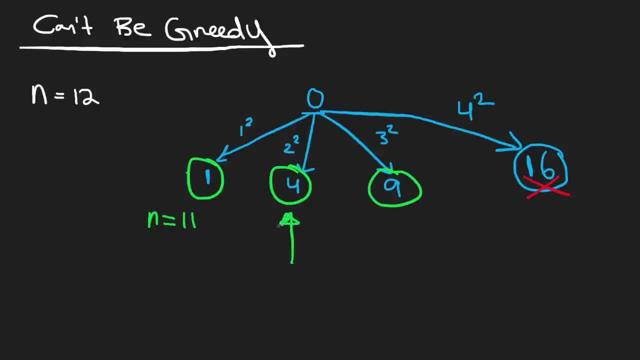 to get to 11.. For this one, we want to know what's the minimum number of perfect squares. does it take to get to eight, right? Because four is going to lead us to 12.. For this one, we want to know what's the perfect number of squares. 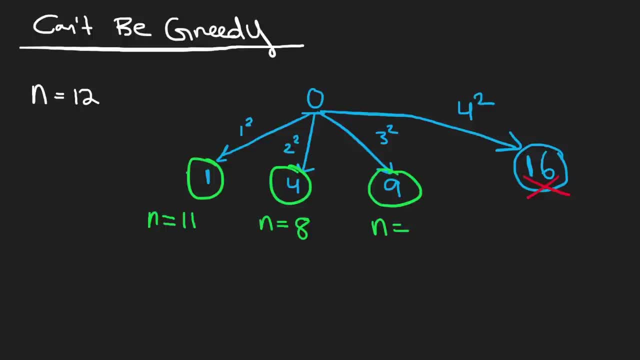 does it take to get to three? So, basically, we're taking this big problem- n equals 12- and breaking it down into three sub problems, right? So whichever one of these yields the minimum number of perfect squares, that's going to be our solution, And so what we're going to be doing here is we're going 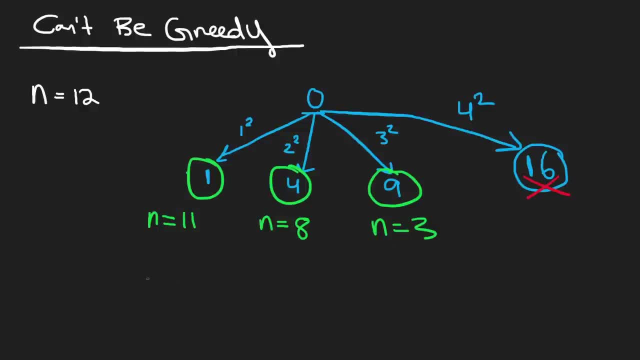 to continue to be breaking these down into sub problems until we get to the base case, which, of course, is going to be equals zero. right? how many perfect squares does it take to sum to zero? of course, that's going to also end up being zero. so what we're going to do is we're going to start bottom up, because we see. 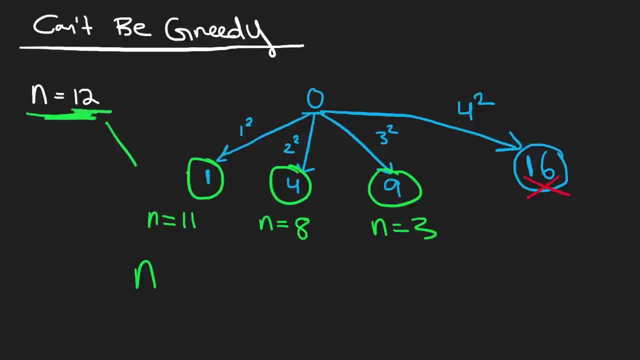 that a big problem like 12 is going to depend on smaller sub problems like 11, 8 and 3. we don't know which ones it's going to be. it could be any of them that are smaller than n. so anything less than n and even 3 is also going to have sub problems, right? so before we want to solve n, 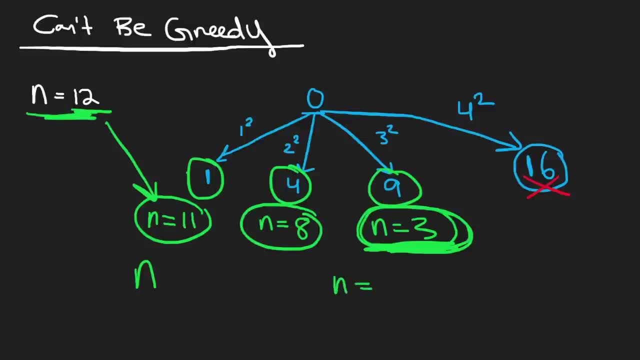 equals 3, we're going to need to solve n equals 2, n equals 1, and the base case is just going to be n equals 0, which we don't need to solve. so this is going to be the bottom up approach. what i'm 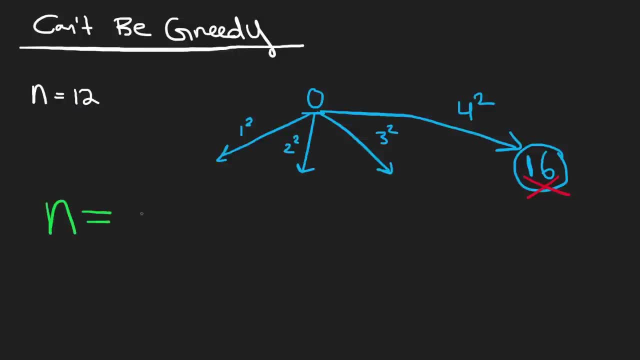 going to be doing is: i'm going to be computing the minimum number of perfect squares, starting at n equals 1, then going to 2, then going to 3, until all the way we get to 12.. and for each of these sub problems, right, let's say, instead of doing 12, we were doing n equals 5. 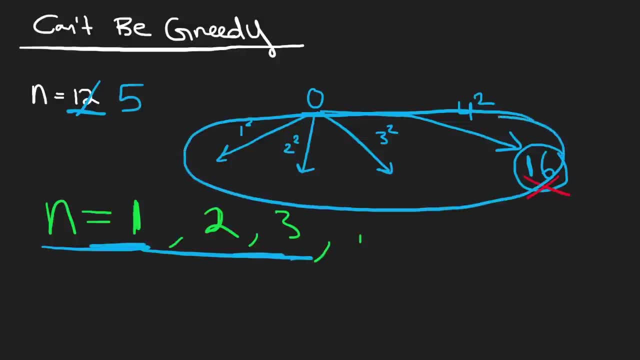 i'm going to make this same kind of decision like i'm going to make. i'm going to try every single possible perfect square. so 1 square, 2 squared, just just like how we stopped early here, like once we got to a number- 16 that was bigger than our n- that we were looking for. that's how we're. 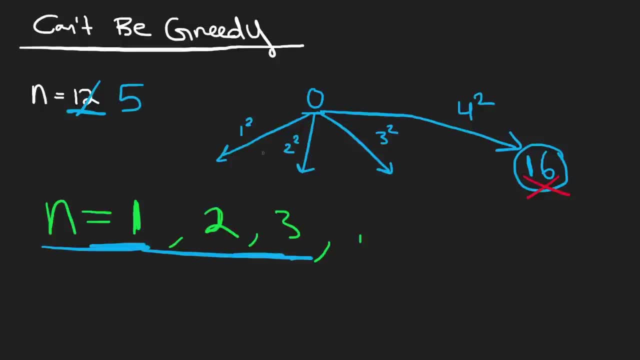 going to stop for the sub problems as well. so, for example, 5. we see that 1 squared is going to be 1. 2 squared is going to be 4. 3 squared is going to be 4. 3 squared is going to be 4. 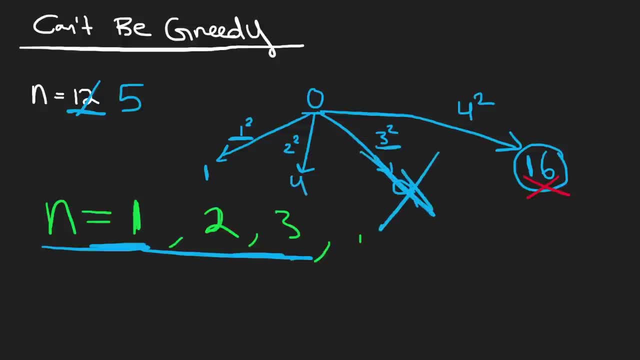 3 squared is going to be 9, so we're going to stop early here. we're not even going to get to this 4 squared 16 position. so, with that being said, what's going to be the time? complexity of this, because we can tell that there's going to be a nested loop. right, we're going to be going, since we're going. 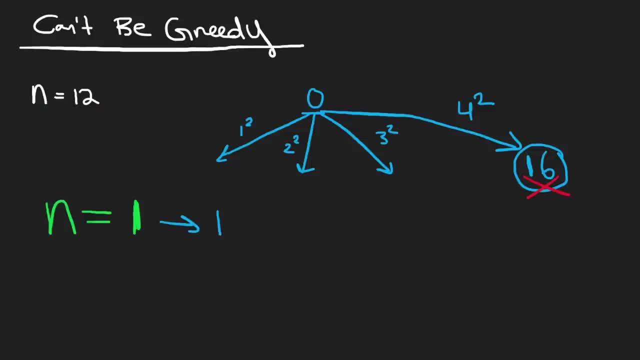 to be starting at 1 and going all the way to n, which in this case is obviously 12. so that's going to be big o of n right, and for each of these n values we're going to have this original layer, like this first layer of the decision tree, or 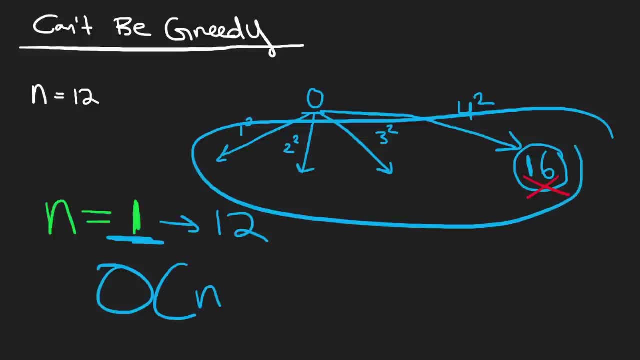 only a single layer, right. but how big is this layer going to be? well, it depends on the value n, right? but we know it's definitely bounded by at least the square root of n, right? because, remember, we're stopping once we get equal to or greater than our n value, right? so we're going to start at. 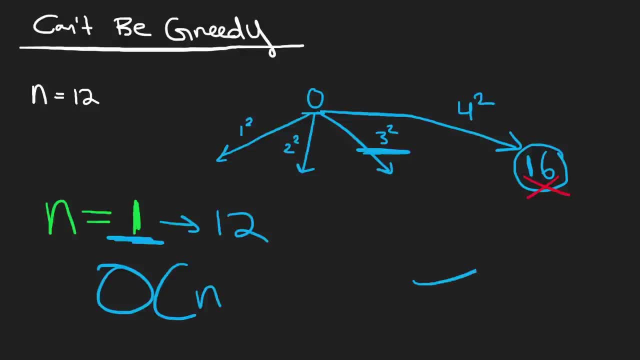 1, then go to 2, then go to 3, and eventually we'll get to either the square root of this, right. in this case, 12 doesn't really have a square root integer. it'll be 3 point, something right. but for example, if, if, instead of being 12, this was 16, we 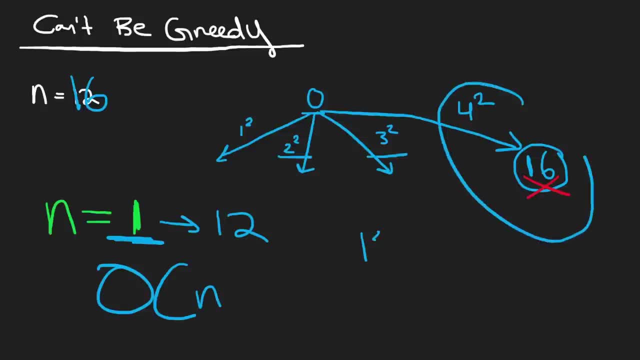 would do: 1 squared right, 2 squared, 3 squared, 4 squared, which is exactly 16, and then we would stop right. so we're stopping at this value, which is the square root of 16, right? so this, the overall time complexity, is going to be bounded by n times, the square root of n. with that being said, let's. 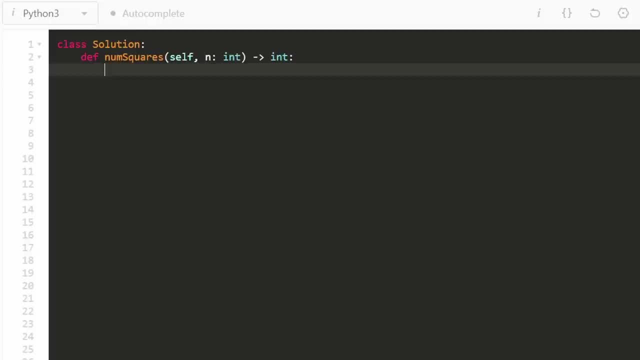 jump into the code. it's pretty short. so we're going to be solving all these sub problems before we solve the original n problem. so i'm going to have a dp array where we store the result of those sub problems. i'm going to initialize every value just to n. you could do max integer if you wanted, but we know that for n. 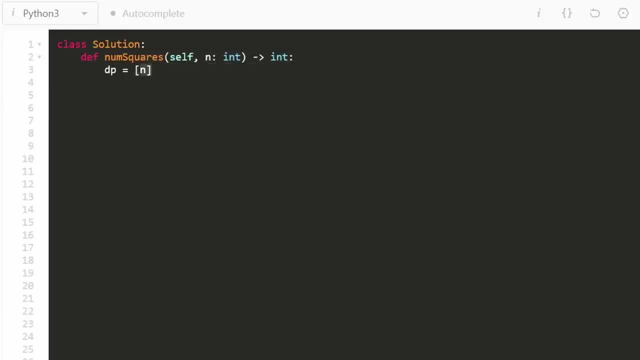 the max number of possible squares is is going to be at the at most n, because you know, at the very least we could do 1 squared plus 1 squared plus 1 squared and then eventually get to that sum, and that we're looking for that target value. 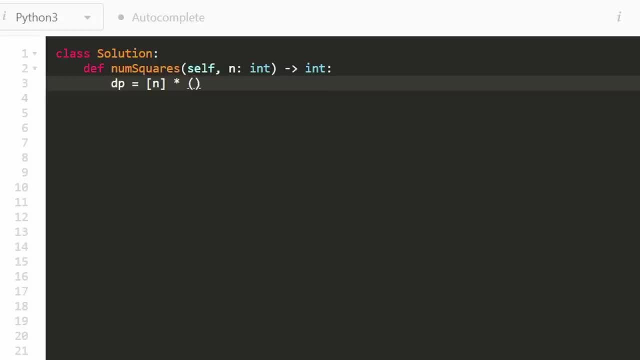 and so the size of this is going to be. we're going from 0 to n, so the size is going to be n plus 1, and remember, the base case is going to be where the target value is 0. we know that that takes 0 squares to. 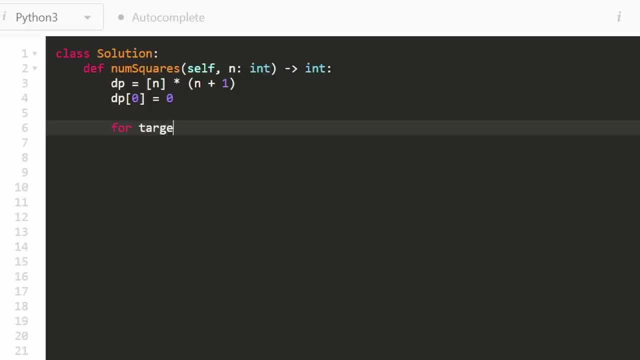 get to that target value. so we're going to be iterating through every target value in the range of 1 all the way to n in python. n plus 1 is non-inclusive, so this is going to stop. the last iteration is going to be n and we're going to be going. 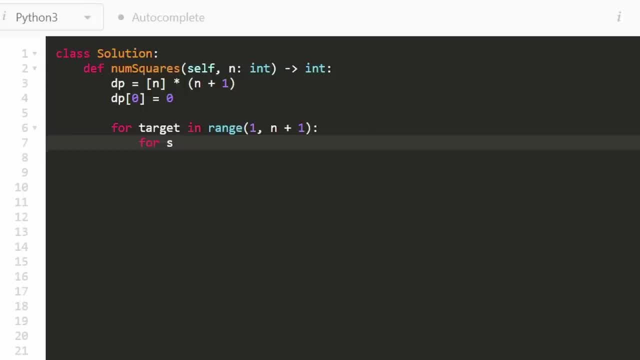 through every single possible square value, so s in range from 1 to the target value plus 1 because this is non-inclusive. this is not the actual square value. this is just we're going through every value from 1 to the target, but we're going to be using s to compute the square, so s times n. 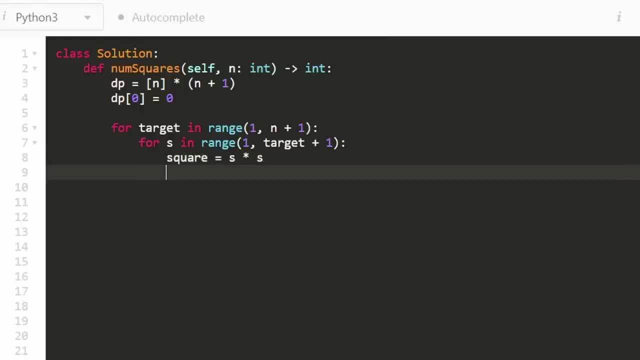 is going to be the square right. we're going from 1, 2, 3, 4. but we know if we go over, for example, if subtracted by the square is less than 0, that's when we're going to break right. that's when we 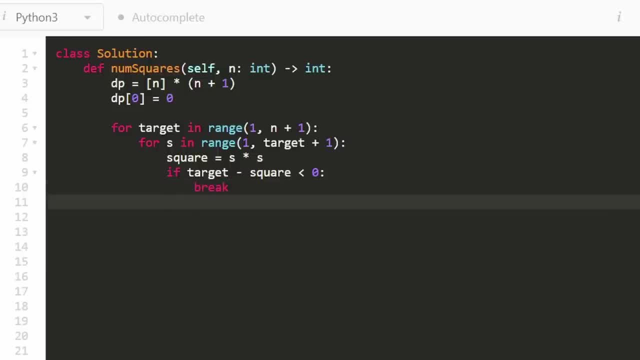 can stop early, we can stop short, we don't need to continue, we don't need to waste our time. but if we don't stop short, that's where we're going to compute the possible solution. so we're going to say, for dp of target, a possible solution could be the minimum of what it already is right. 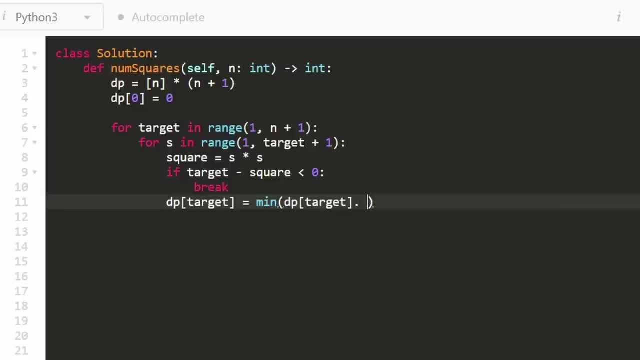 in that case there would be no change, or the minimum of the remaining amount. so, for example, target minus square: right. so let's say our target was 12, our square was 4. now the new value that we're looking for is 12 minus 4. so we're looking for 8, right, so we're 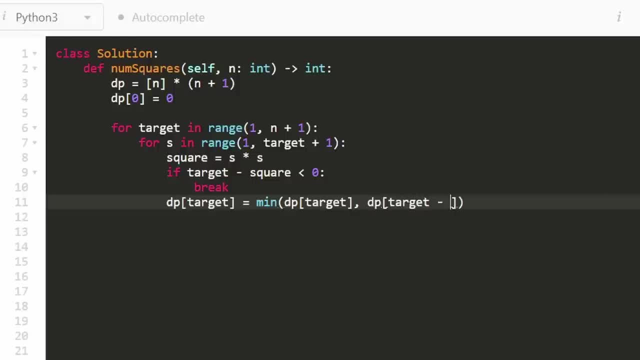 going to say dp of target subtracted by square right. that's why we're solving this from 1 all the way up to n, because we're depending on the smaller results. that's why it's called bottom up, because we just used a square. remember, what we're trying to do is counting the number of minimum. 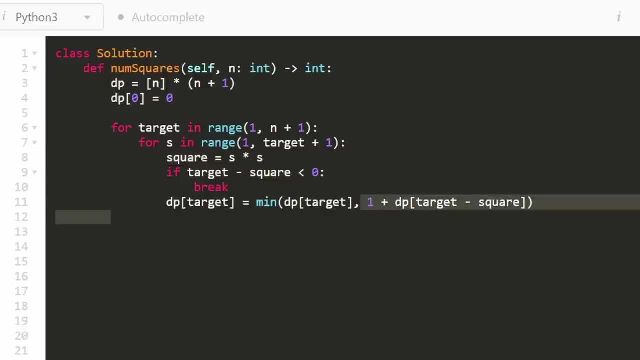 squares. we just use a single square, so 1 plus. whatever the minimum number of squares it takes to compute this new amount right- 12 minus 4- how many minimum squares does it take to get to 8 plus? you know the single square that we just used right now, and once that is done we'll have gone. 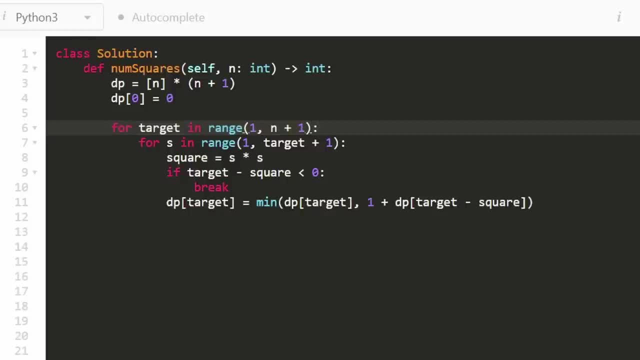 through every single target value, 1 all the way to n. so therefore the the solution to n will be stored in our target value and we're going to be able to compute the number of squares that we have in our dp array. so then we can just return that return dp at position n. that's going to be. 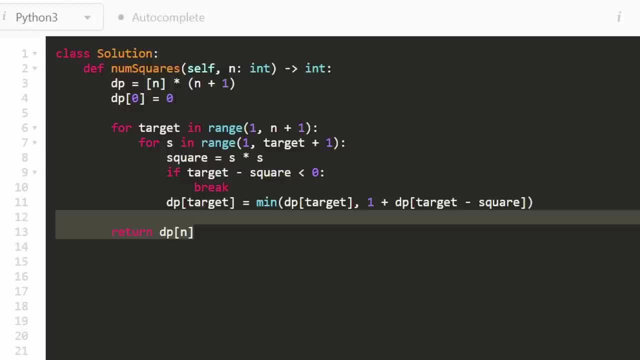 the minimum number of squares it takes to get to n. so remember the overall time complexity of this is big o n multiplied by square root of n. you can kind of write that like this. there's not a good way to do it, but yeah, that's the time complexity. there is a more efficient way to solve this. 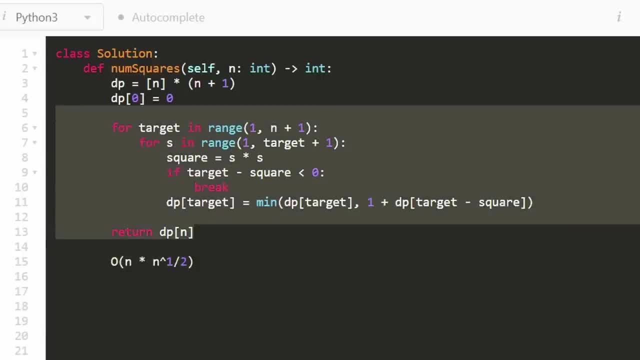 problem, but this is kind of the main solution that I think an interviewer would look for like this is the actual intuitive solution. there are some more mathematical solutions that I don't know. if you know, that would actually be helpful to learn, but I hope that this was helpful. if it was, please like and subscribe it supports. 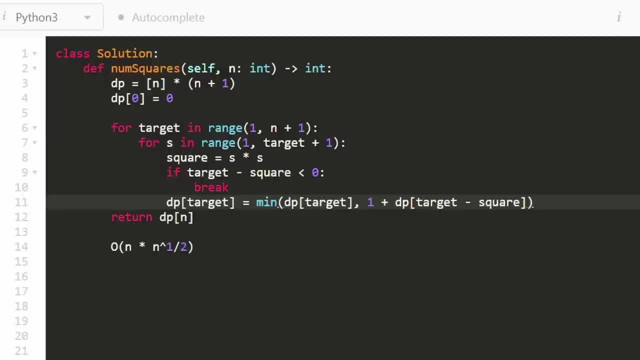 the channel a lot and I'll hopefully see you pretty soon. thanks for watching. 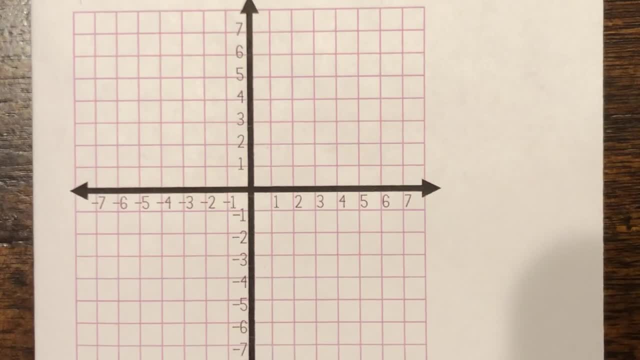 We're still working with polygons on the coordinate plane. Today we're going to do a little more practice with plotting those on the coordinate plane and identifying what shape it is that we're plotting and then finding the area of that shape. So let's go ahead and do chapter nine. 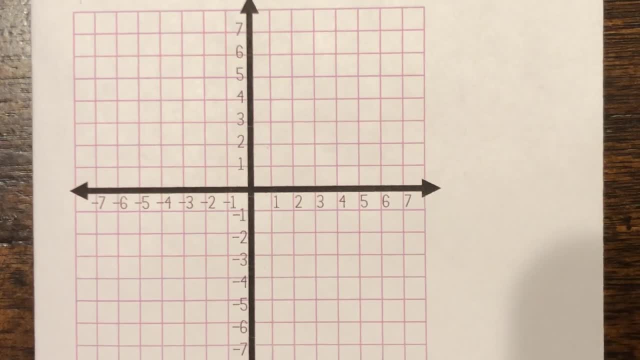 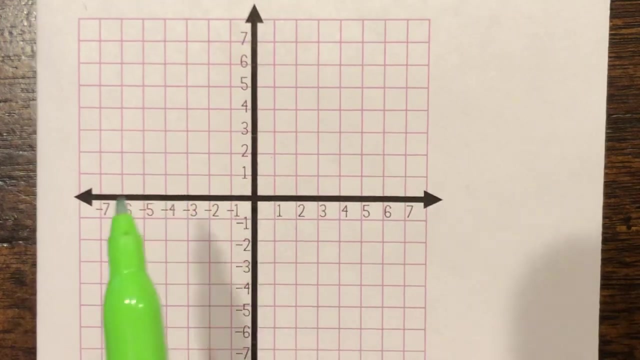 lesson five, extra practice number five, And this question says: graph each figure and classify it, then find the area. So first let's go ahead and start graphing these points. First we have negative four, four, And remember on our coordinate plane we need to walk before we take our. 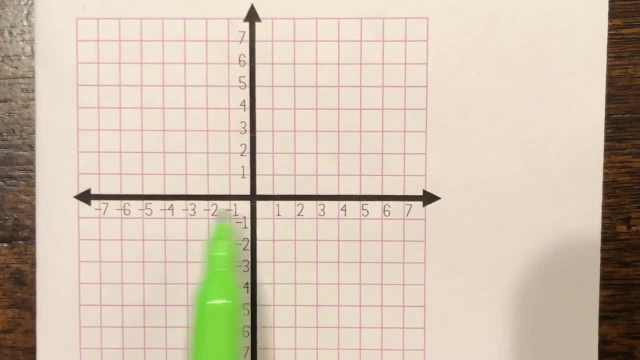 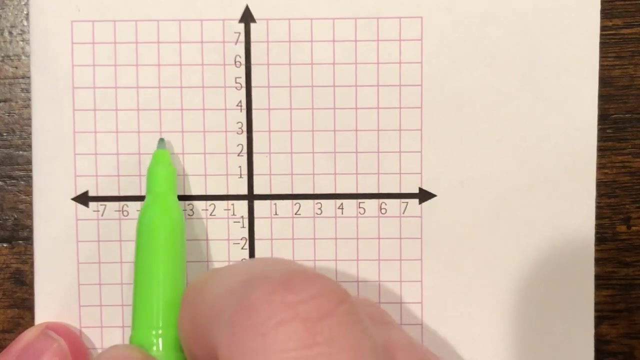 elevator. So if we have negative four, we're going to go to the left. negative four, because negative is left and down and positive is right and up. So we're going to go negative four, two, four, four. So we're going to ride the elevator up. One, two, three, four, Okay, And this is point A.